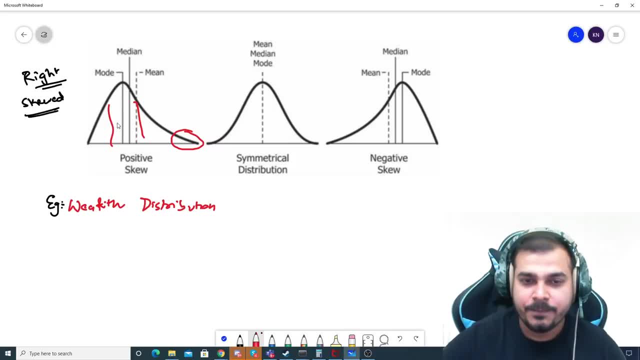 will be finding people with the same amount of wealth, Right? This is one classical example. The second classical example that I would like to take is probably you, can you know that, like you have seen my channel- you have seen most of my videos, guys- you'll be seeing that some of the people like to write a longer comments, right, probably after seeing a video. So length of the comments, length of comments, probably in my video, this is also a classical example, Right? So here you'll be seeing 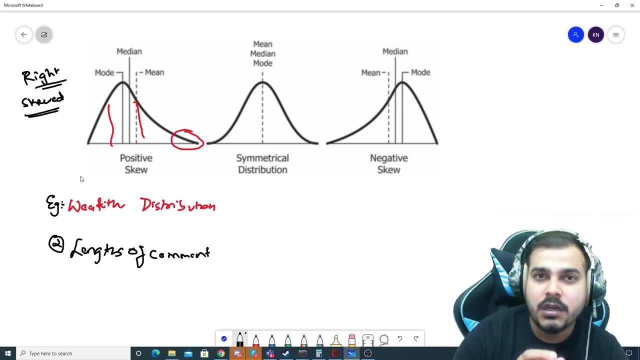 that some of the people will be writing longer comments. They are also some of the people who will be writing smaller comments and some of the people will. most of the people will be writing medium sized comment, probably one liner, Right? So this is two classical examples that I want to give. Yes, in the morning video, many people gave some amazing examples- itself Right, And you should also check out that Again. the link will be given in description. Now, coming to the second distribution, second distribution, which is called a symmetrical distribution. This is nothing but our normal distribution. This is the example. 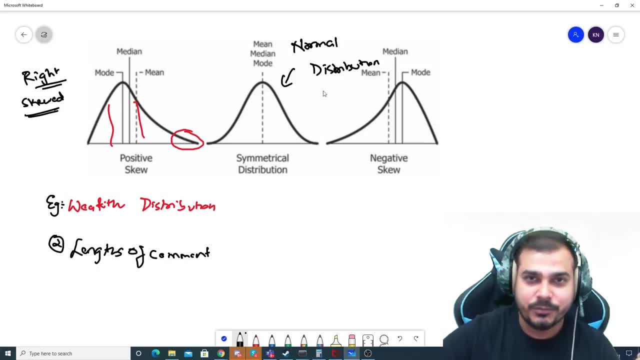 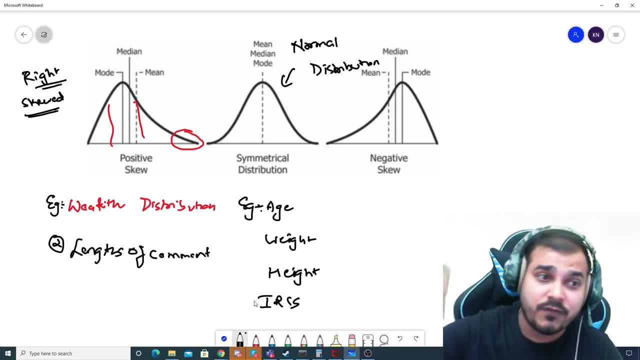 Petal weight, sepal length and sepal weight- Right, That was also falling- this kind of normal distribution. And remember, guys, most of the machine learning algorithm likes the data to have this kind of normal distribution property, And why it is called a symmetrical distribution, Because the right hand curve will almost be equal to the left hand curve. Okay, So these are like mirror face. Fine, Coming to the third kind of distribution, which is also called as left skewed distribution. It is also called as negative skewed distribution. Here the left hand side will be a little bit. 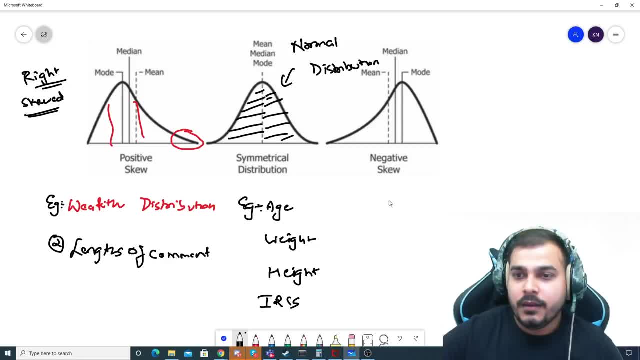 elongated. and then the right hand side, Right. So here the perfect example. I'll say lifespan of human being. Lifespan of human being, Because there are many people. if I talk about the average lifespan, it is somewhere around 50 to 70. So 50 to 70 will basically be falling in this particular region. There will be people who will be dying quite early in the age, but there will be also very less number of people who will be living. 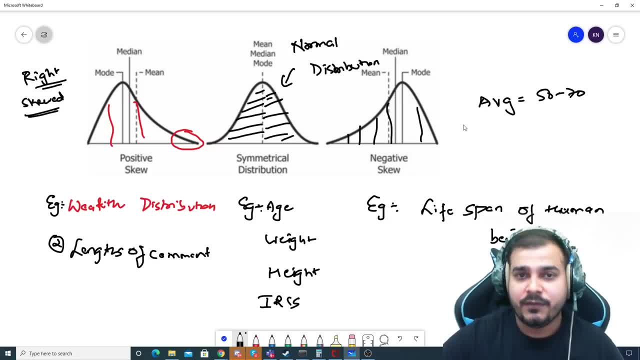 more than 70 years, probably near 100, and all Again, a perfect example to make you understand. Yes, if you have some more examples, definitely. many people had also written in the morning And I like most of the examples itself Right Now. coming to the second question: what is the exact relationship with respect to mean, median and mode? It is very, very much simple. Just by seeing this particular diagram, I think you'll be able to know it. guys. Mean in the right skewed distribution over here will be greater than median And median will be greater than median. 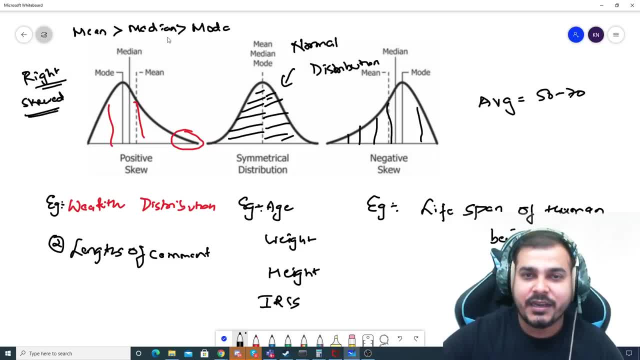 And median will be greater than mode, Right? So mean will be greater than median And median will be greater than mode. So this is the exact relationship that you'll be able to find. Just by seeing this particular diagram, you'll be able to understand. In the case of symmetrical distribution, mean will be approximately equal to median. It will be approximately equal to mode. So this is the second relationship that you find out with respect to normal distribution. The third one, basically what you see over here. if I take this particular example over here, your mode is 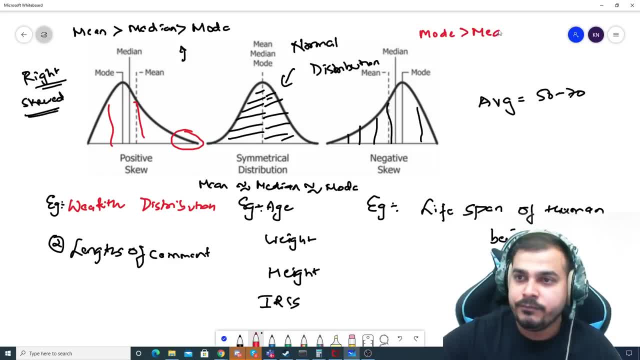 highest, then your median, then your mean, Right. So this is the exact relationship. Let me just write it down if you are getting confused. First the highest will be mode, then your median- you have, because median will be obviously smaller than mode- then you have mean. So this is the relationship that you find out with respect to the negative skewed data. So this is what the interviewer may.